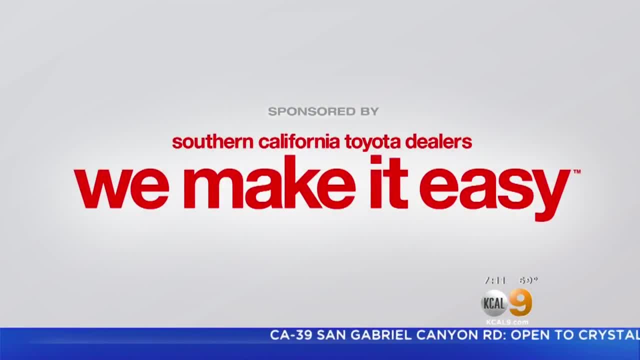 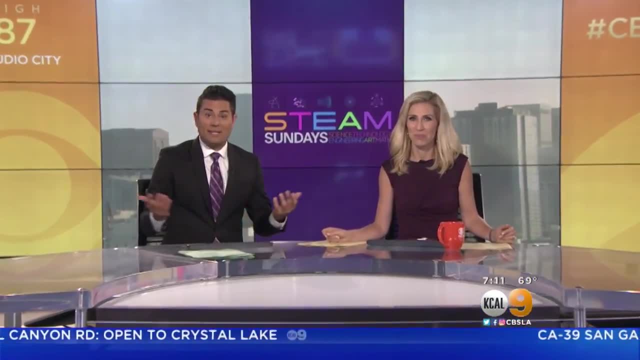 STEAM SUNDAYS, CHAMPIONED BY YOUR SOUTHERN CALIFORNIA TOYOTA DEALERS. OKAY, SO TALK ABOUT A DREAM JOB. HE PLAYS IN THE SAND. HE MAKES MONEY DOING IT. 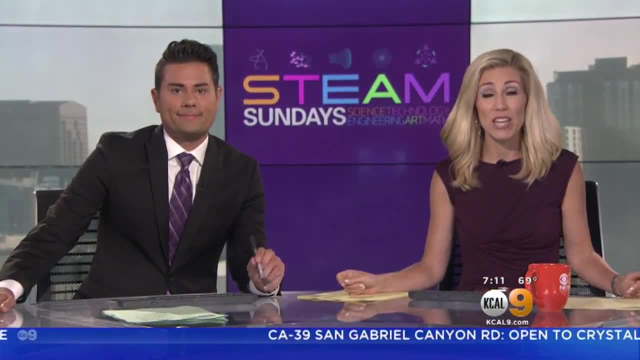 IT'S TIME FOR THIS WEEK'S STEAM SUNDAY PROFILE. KCONI METEOROLOGIST AMBER LEE INTRODUCES US TO A NEWPORT BEACH ARCHITECT WHO'S MASTERED THE SCIENCE OF SANDCASTLE BUILDING. 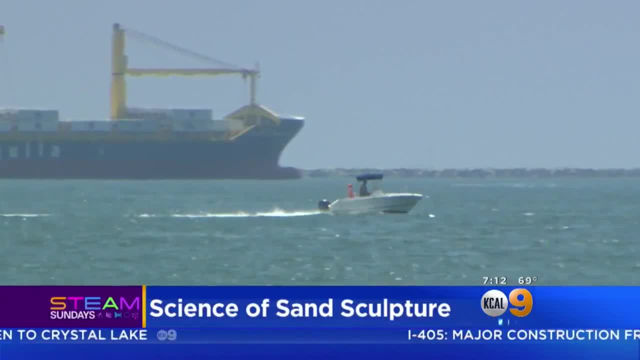 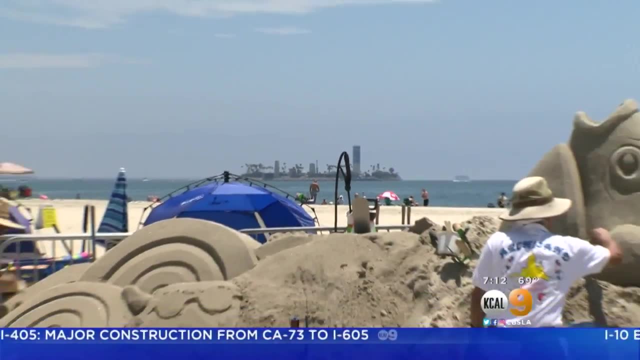 WE'RE SOAKING AND COMPACTING THE SAND. ANOTHER SUNNY DAY IN LONG BEACH. ANOTHER MASTERPIECE AWAITS ITS EVOLUTION FROM A SAND PILE. BY THE END OF THE DAY, THIS MOUND WILL BE UNRECONNIZABLE. 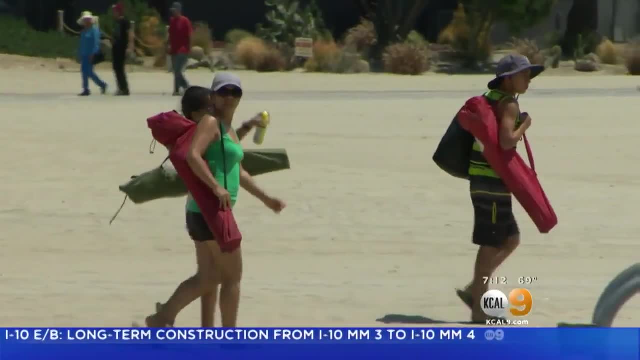 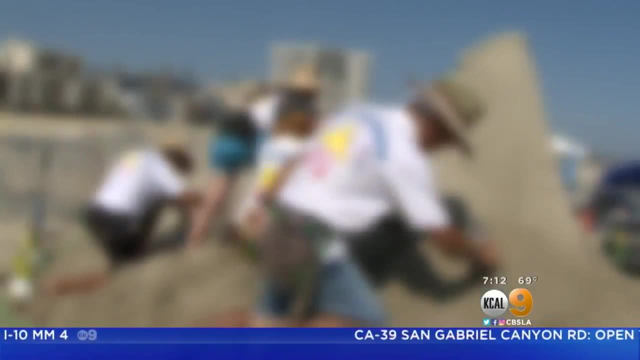 ITS MISSION TO BECOME A FISH HOLDING A SURF BOARD. THAT'S RIGHT. THIS WILL BECOME SOMETHING. RESEMBLING THIS, WE TOOK THE TOYOTA MOBILE WEATHER LAB OUT TO SEE HOW IT HAPPENED. 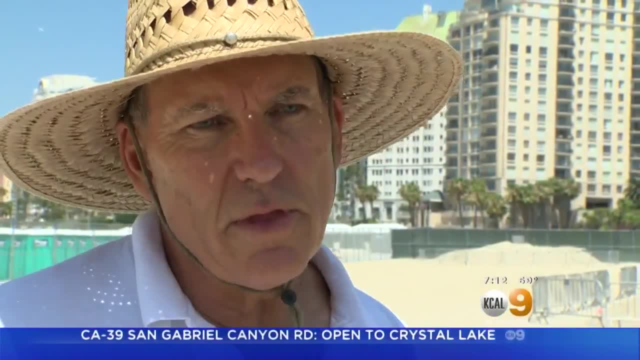 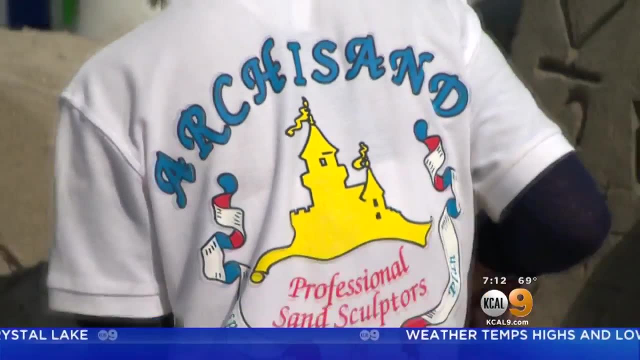 MY LIFE HAS BEEN A LONG TIME. I'VE BEEN DEDICATED TO BUILDING THINGS, WHETHER THEY'RE PERMANENT OR TEMPORARY. MEET GREG LEBON, PRESIDENT OF ARCA SAND IN NEWPORT BEACH. 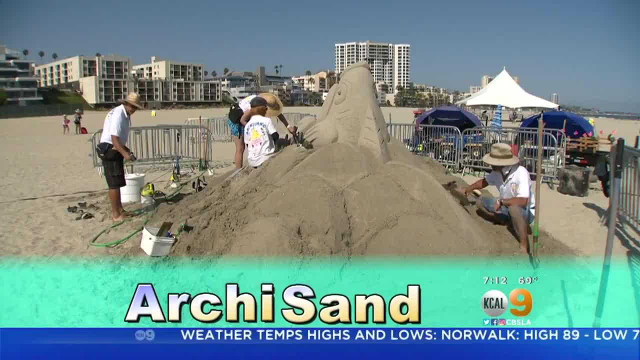 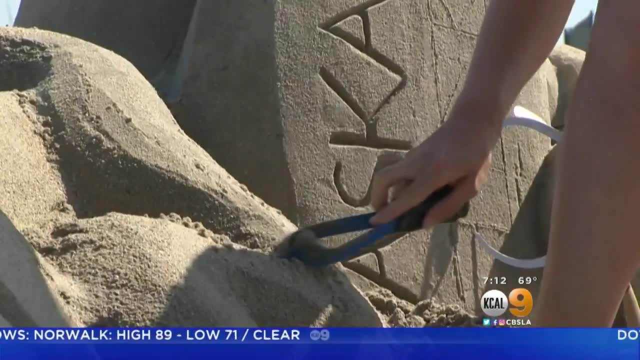 ARCA AS IN ARCHITECTURE, SAND AS IN THE STUFF COVERING OUR BEACHES. WE CREATE SAND SCULPTURES TO PROVIDE JOY AND AMUSEMENT FOR THE PUBLIC. GREG'S PORTFOLIO IS PRETTY MIND-BLOWING. 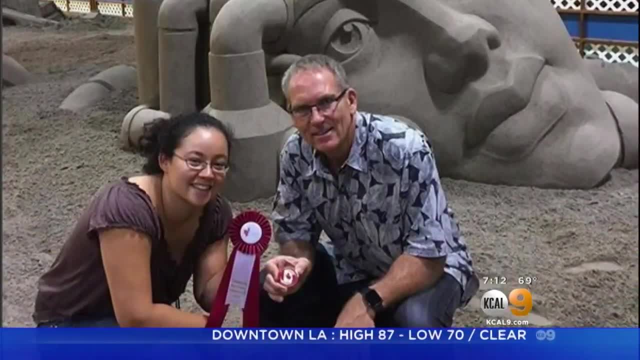 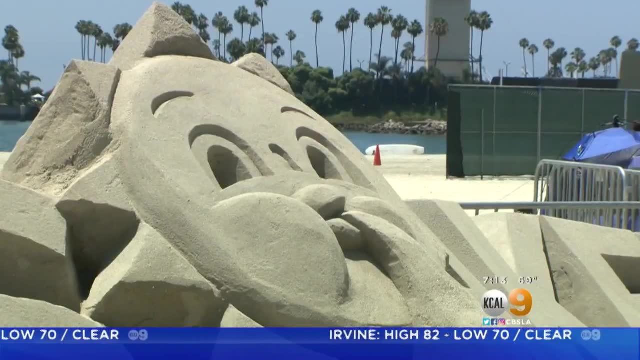 OVER THE PAST 40 YEARS, HIS SCULPTURES HAVE WON COMPETITIONS ALL OVER THE WORLD. HE'S BUILT SAND CASTLES, SKELETONS, CELEBRATED THE SUMMER OF LOVE AND RECENTLY WELCOME GUESTS TO THE SUN-SOAKED FESTIVAL. 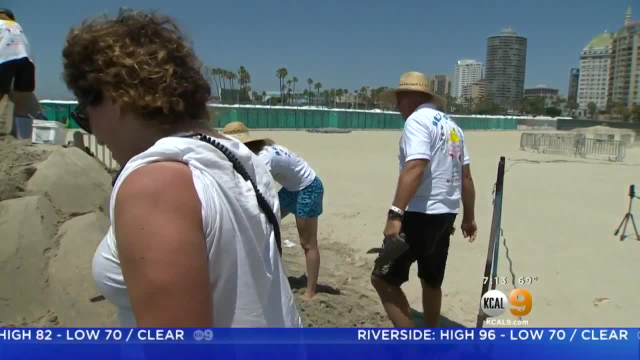 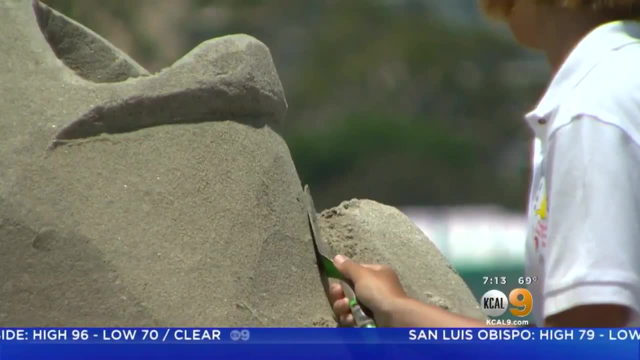 THIS IS THE PROCESS THAT MAKES THE DIFFERENCE TO DO WHAT HE AND HIS TEAM DO. WE HAVE TO UNDERSTAND THE SAND, WE HAVE TO UNDERSTAND ITS STRUCTURAL CAPABILITIES AND ITS LIMITS, AND THAT'S WHERE THE STEAM DISCIPLINES COME INTO PLAY. 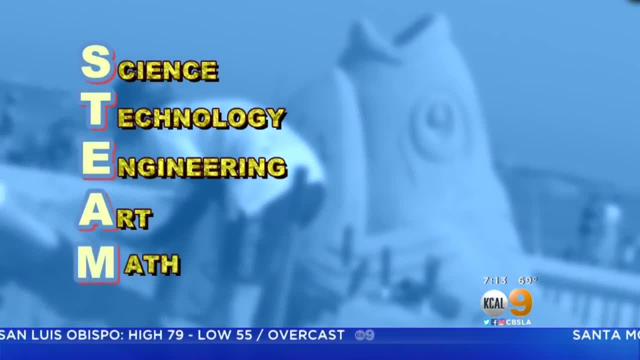 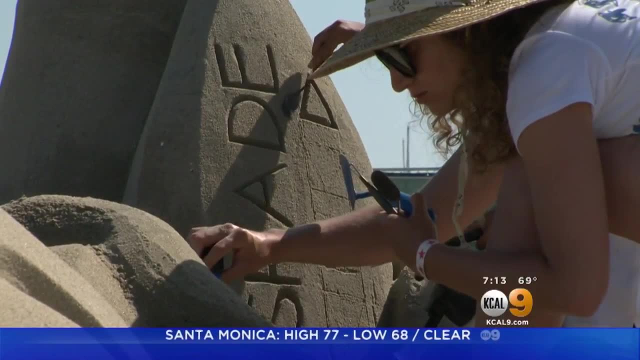 SCIENCE, TECHNOLOGY, ENGINEERING, ART AND MATH. I'M GOING TO SAY WE PROBABLY EMPLOY A VARIETY OF ALL OF THEM, THE THREE DISCIPLINES MOST IN USE HERE ON THE BEACH. 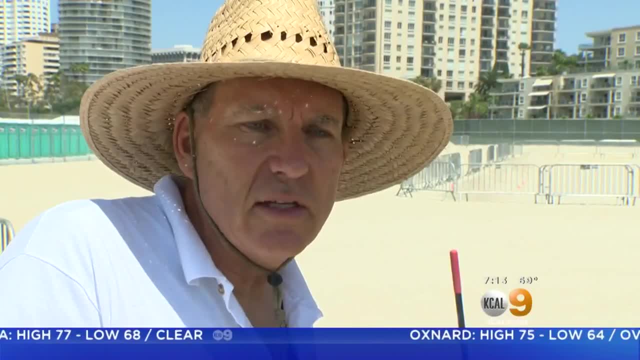 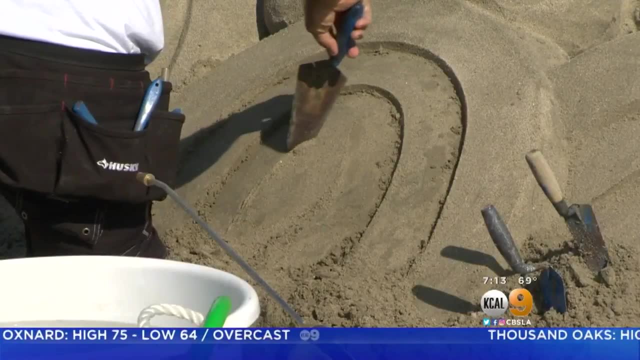 SCIENCE, ENGINEERING AND ART. THERE'S SCIENCE, AND UNDERSTANDING THE SAND. THE ENGINEERING IS ESSENTIAL TO CREATING SCULPTURES THAT CAN HOLD THEIR SHAPE, AND THEN THERE'S THE ART, PART OF IT, WHICH IS OBVIOUS.